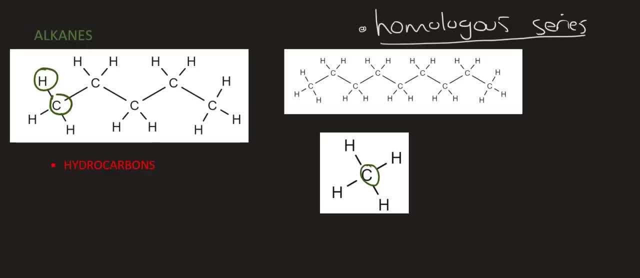 is homologous, So homologous is a type of homologous series. So we are looking at the alkanes, which are a type of homologous series. You get other types like alcohols, ketones, aldehydes, but we're looking at alkanes. Okay, so they are hydrocarbons. They also have some. really, 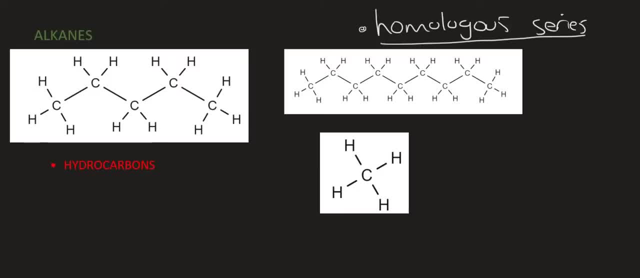 cool thing happening. Check this out: If you count the number of carbons in this first molecule, there are 1,, 2,, 3,, 4, 5.. Then, if we count the hydrogens, there'll be 1,, 2,, 3,, 4,, 5, 6,, 7,, 8,, 9, 10,. 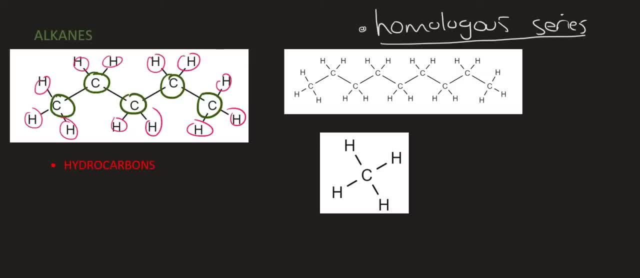 11, 12.. Okay so, Kevin, what's so cool about that? Well, I'm just going to write that down for now. So I'm going to say that there are 5 hydrogens, and I mean 5 carbons and 12 hydrogens. Let's do. 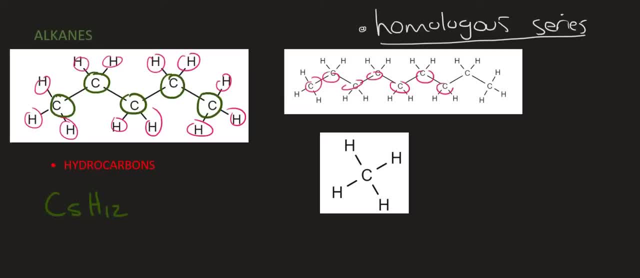 the next one. So there's 1,, 2,, 3,, 4,, 5,, 6,, 7,, 8, 9 carbons, And then I'm not going to waste my time, But if you had to go count all of those hydrogens, you'd see that there are 20.. Don't believe me. 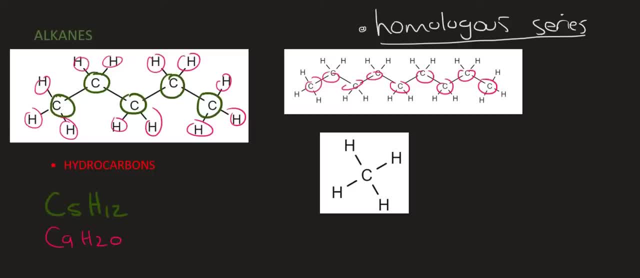 Pause the video, check it out And so we can see that we have C9H20.. Then this one over here has 1 carbon and 4 hydrogens. Now there's a pattern emerging. I know it might not look really obvious. 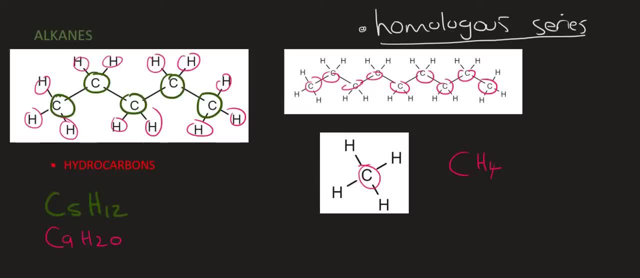 right now. but check this out. The pattern is the following: If you times the number of carbons by 2 and then you add 2, you will get the number of hydrogens that they are meant to B. So, for example, if there are 9 carbons, if you times that by 2, that's 18 plus 2, that gives you. 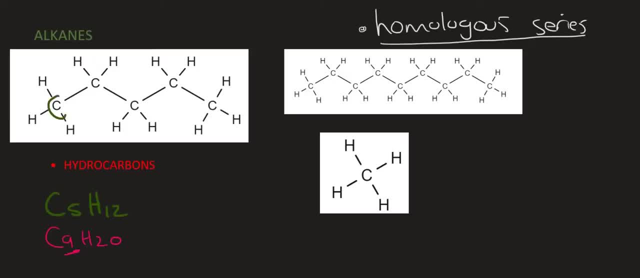 20. And guys, this isn't rocket science. Check this out. For each of the carbons that are in the main chain, they always have 2 hydrogens- like definitely See that. And then the 2 on the end. 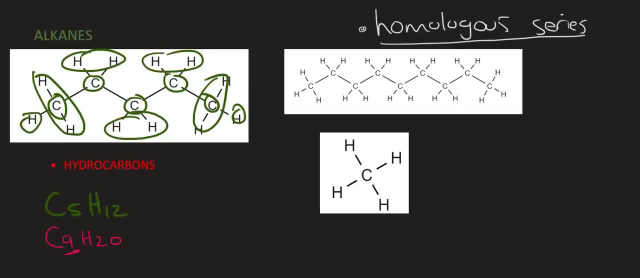 they have an extra one. And that's why I said you can take the number of carbons, multiply that by 2, because that's the number of hydrogens that they have- And then you can just add 2 to the answer for the 2 hydrogens that are on the end, And so we can say that the general 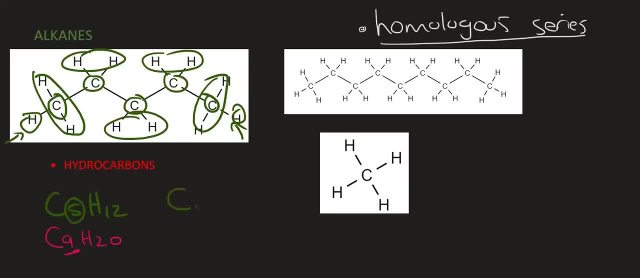 formula for hydrocarbons or for alkanes will be CnH, then you say 2n plus 2.. So if we have 10 carbons, then you say C10, and then the Hs will be 2 times 10 plus 2.. So that will be H22.. And so 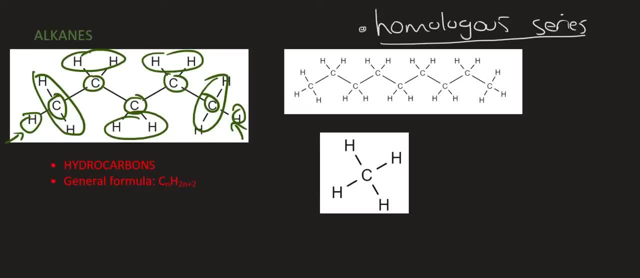 there we have it, guys. The general formula is CnH2N, And then you can just add 2 to the answer, N plus 2.. So you need to get used to that, because I could, for example, in an exam. 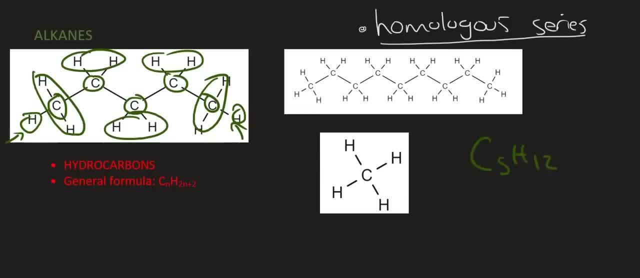 they could say: OK, so we've got this molecule C5H12.. Give the homologous name. Now you might say alcohol, aldehyde. But if you realize, hey, hey, it's only got carbon and hydrogen. 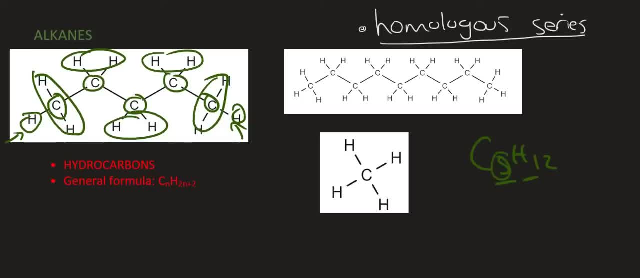 so that could be an alkane. And the ratio is 2n plus 2.. So you say 5 times 2, which is 10 plus 2 is 12.. Oh, that's an alkane, All right. So here's a very random question: What do we use a towel for? 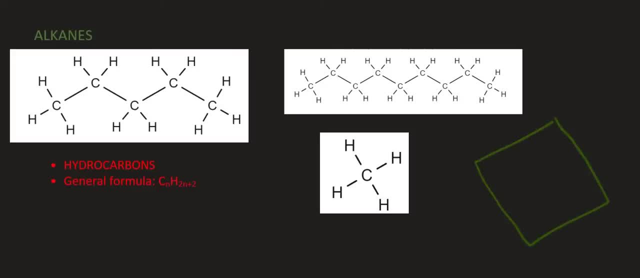 You know a towel that you use when you get out the shower, out the bath. That towel is used to soak up water from your body. OK, But let's say you're working in the kitchen, for example, and you spill a huge bucket of water all over the kitchen floor. 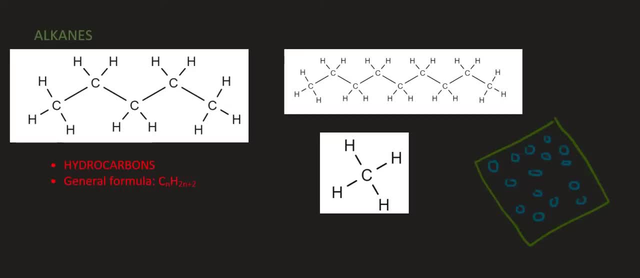 because we all work with buckets of water in the kitchen, don't we? Now, if you were to use a towel to try and clean up that water, or try to soak up that water- I'm sure you've done this before- You'd realize that that towel does not. 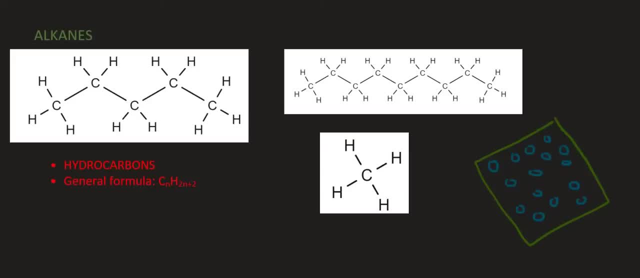 have enough. what could we call it Water retaining ability? OK, It can't collect all the water. Eventually the towel becomes full, or- the proper scientific word- is saturated, and then you can't add any more water to that towel. That's usually when you'd have to go squeeze the towel so that 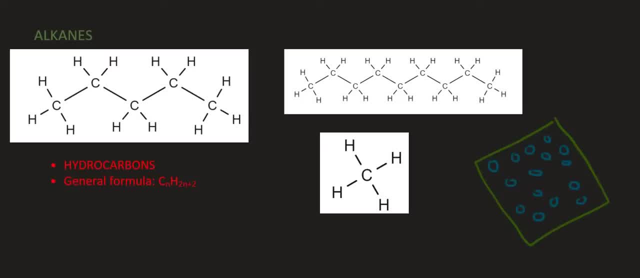 all the water comes off, And then you could use the towel again to try soak up some more water. So in chemistry we're going to talk about the word saturated, And when something's saturated, it means you can't add anything more to it. So what I want you to do is quickly look at each of. 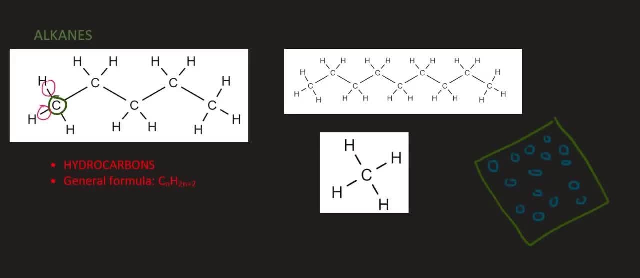 these carbons? They have one, two, three, four bonds. I can show you any of them, Check here: One, two, three, four, And so those carbons are saturated. We know that carbon can only form a maximum of four bonds, And so alkanes are saturated. We will look at alkenes next. 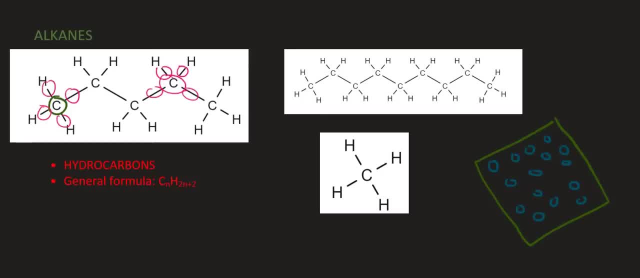 and we'll see what unsaturated means. OK, so the next important thing you need to know about alkanes is that they are saturated, And that's about it really. We'll look at alkanes at a later stage when we start looking at the naming, But for now, those are your alkanes. I hope you're. 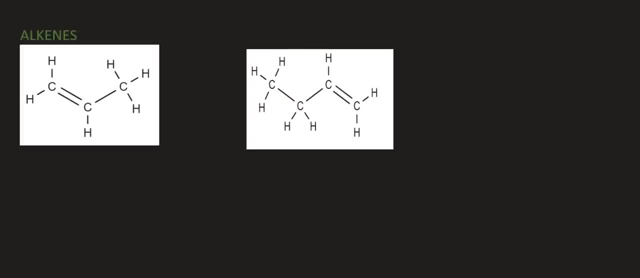 feeling a lot more comfortable with them. Next will be the alkenes. Now, the alkenes are the guys that have the double bond. OK, that's what's important for them. So this will be a lot faster than the alkanes, because straight away we see that there's only carbon and hydrogen, And so 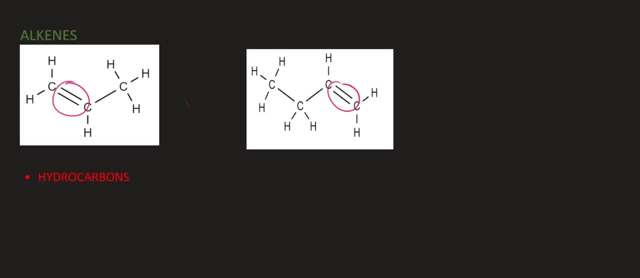 these are also called hydrocarbons. And, guys, the word hydrocarbon, it's self-explanatory: Hydro for carbon, for carbons, There's only hydrogens and carbons. Aha, Next we need to look at their. 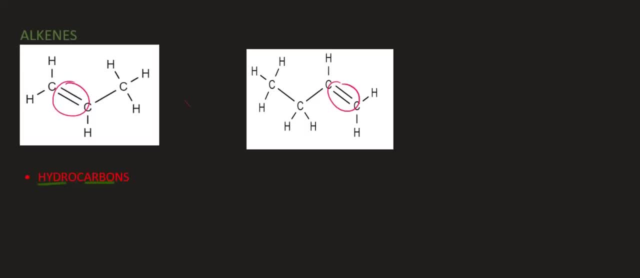 general formula. Oh and, by the way, their homologous name is alkenes. OK, so remember that is a type of homologous name or homologous series. I know it's a weird word, homologous Who? 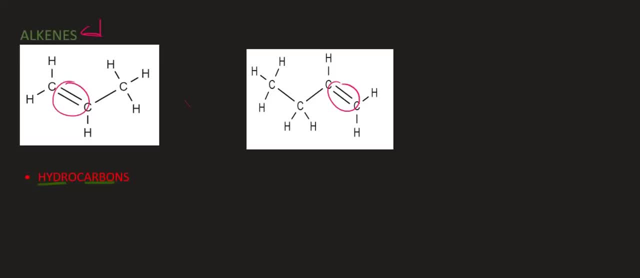 comes up with that. But that's the group of molecule. It's called the alkenes. OK, and remember, there's nine different types, nine different homologous series. Let's look at the alkenes. So if we look at this first one, it's got one, two, three carbons. OK, so I'm going to say 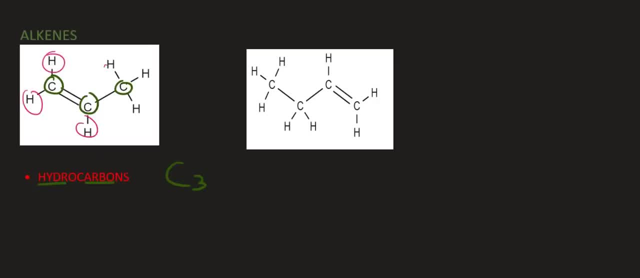 C3. Then if you count the hydrogens, there would be six. For the next one, one, two, three, four carbons. And if you count the hydrogens, one, two, three, four, five, six, seven, eight. OK, so look. 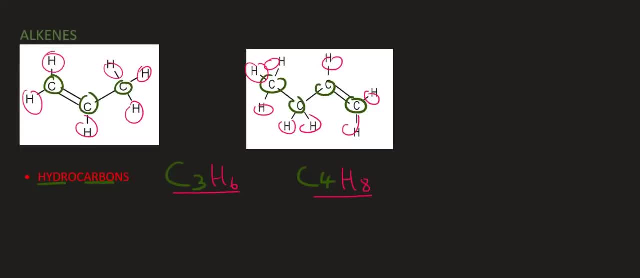 at the pattern now, The hydrogen is always double the number of carbon. So let's see how this makes sense. These alkenes are the same as alkenes, but they have a single double bond. OK, Oh, by the way, if an alkene has two double 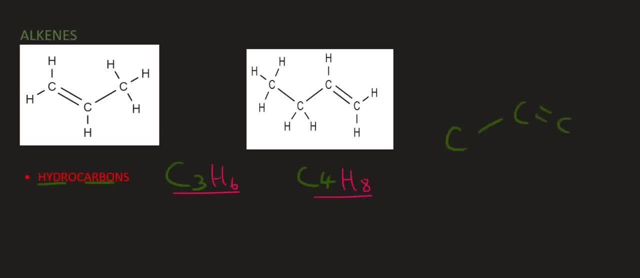 bonds. we haven't looked at something like that yet, but you can easily get a molecule that does something like this. When there's more than one of those double bonds, then these formulas don't work. OK, I've never really seen them do that too much in an exam, But just remember that. 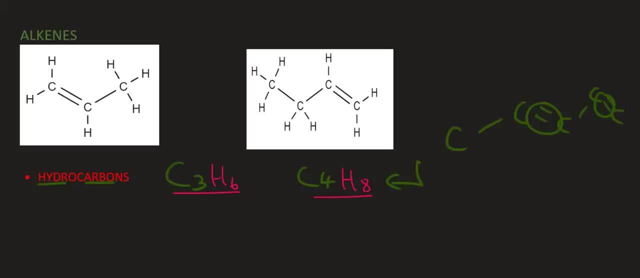 those general formulas only work if there is one double bond. So, as I was saying, these are the hydrogens which have the general formula H times two, N plus two. But we need to understand how a double bond is formed. So if we have a carbon, carbon with hydrogens, OK. so the important thing. 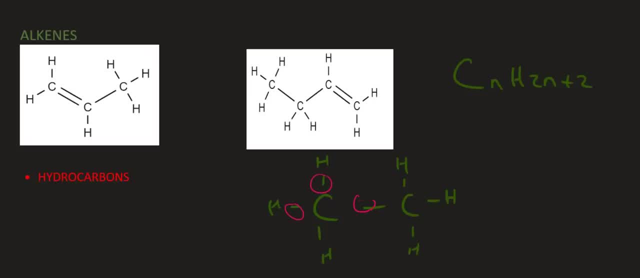 is: look at how many bonds are surrounding each carbon. There is one, two, three, four and then one and then four for that one. Now, that always has to be like that for carbon. So what's going to happen is the following: If we want to form a double bond, we can put a little double bond over. 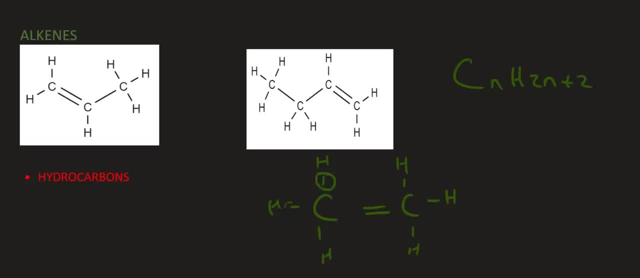 it. Now, if we want to form a double bond, we can put a little double bond over it. Now, each of your carbons have one, two, three, four, five. That double bond consists of two bonds, Hence it's. 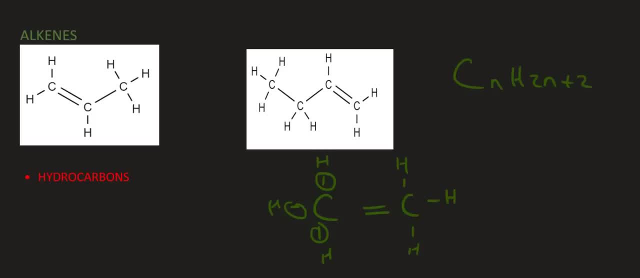 called a double bond. So we have a bit of a problem. So what we're going to do? unfortunately we're going to have to kick away some hydrogens- sorry, hydrogens- on either side. Now have a look at each carbon. So this carbon on the left now has one, two, three, four, So now everything makes 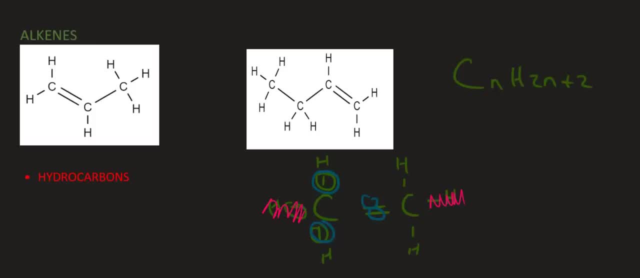 sense, Carbon is happy again. It is bonded to four. Now we're going to have to kick away some four. It has four bonds surrounding it, And so notice what we had to do. We had to knock off those two hydrogens, okay, And so that is why we are going to lose this part, And so this part here. 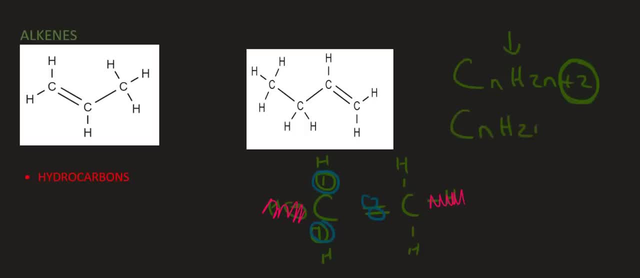 was for alkanes, but alkenes just do this: They lose that plus two, And so that is the general formula for alkenes. Now we need to look at the concept of saturated and unsaturated. These molecules, these alkanes, they are not saturated. That means that they are like a towel. 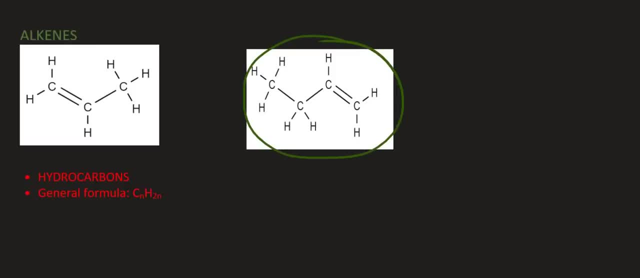 that can still collect more water. The reason I say that is the following: If I had to come along- so I come along here, I come along here and I break this bond over here- then if I enlarge this part of the molecule, it's going to look like this: You've got a carbon and then you've got 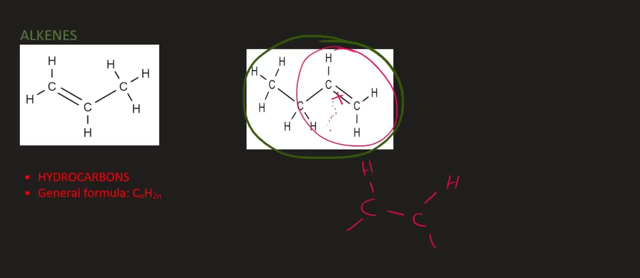 a hydrogen, and then you've got a carbon and a hydrogen and a hydrogen. I've broken one of those double bonds, and so there's only a single bond now, okay, Oh, and then this one was bonded to a carbon. What's happened now is that it's not going to be a single bond, It's going to be a single. 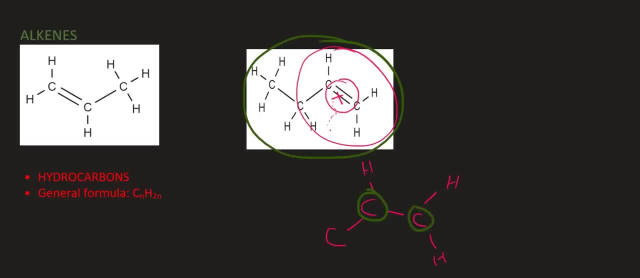 bond. Each of these two carbons are only surrounded by three molecules or three atoms, And so if you break that double bond- which is fairly easy to do in chemistry- you can then, to complete carbon's requirement for having four bonds, you can then add another. 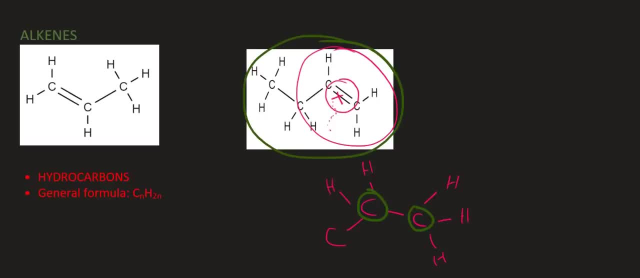 hydrogen. That's like adding more water to your towel. So if you ever see a double bond or a triple bond, you must remember that those are unsaturated, meaning that they can still have more things added to them. So if you ever see a double bond or a triple bond, you must remember that those are unsaturated, meaning that they can still have more things added to them. 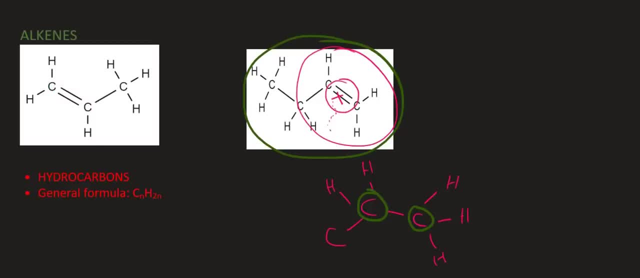 to them Because, once again, if I come along, because over here I can't do anything, I can't break a single bond. A single bond, it's very stable. A double bond, you can break it. So you break this one over here. Now, all of a sudden, this carbon only has three things surrounding it. 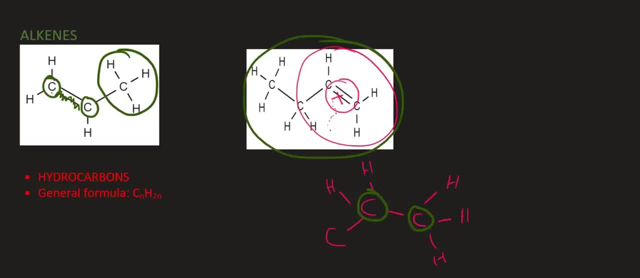 and so does this carbon. So what we can then do to fix that is, we could add a hydrogen to each thing, And so notice that we can still add more atoms to this molecule, and so we call it unsaturated. And lastly, the alkynes. I promise this one's going to go a lot quicker. The alkynes are very 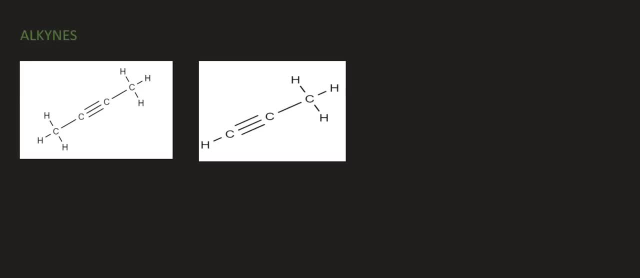 teachers barely ever test these ones, but they are pretty much the same as alkanes, except that they have a triple bond. So it makes sense that there's no hydrogens attached here, Because if I had to attach a hydrogen over here, then if you had to look at. 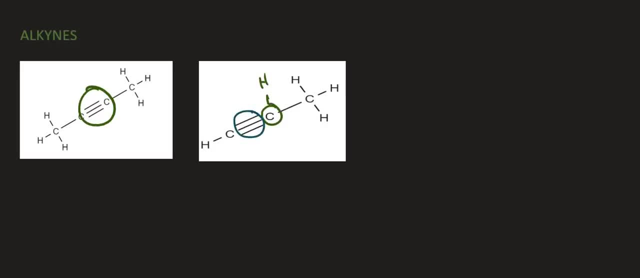 this carbon. it would be surrounded by three bonds, here four and then five. So remember, carbon can only be surrounded by four bonds at a time, not three and not five. So quick summary: they are hydrocarbons, meaning there's only hydrogen and carbon. 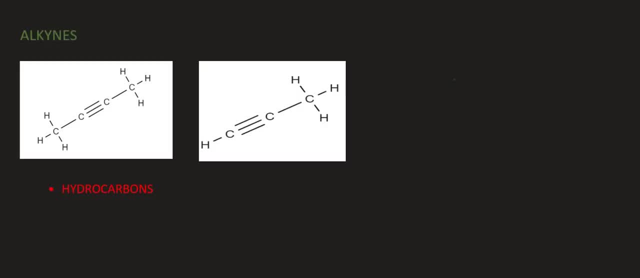 Their general formula. I'm going to go through that, So if we can imagine that these ones have even less hydrogen. so let's quickly look here: One, two, three, four carbons And then, if you quickly count that up, that's going to be six hydrogens, So that's C4H6.. This one here is one. 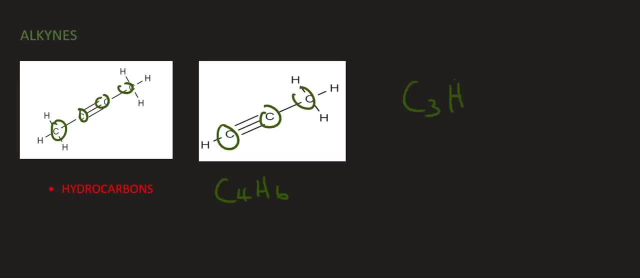 two, three carbons and the hydrogens will be four. The formula for these ones is: you multiply the number of carbons by two, So you multiply the number of carbons by two, and you multiply the number of carbons by two, and then you subtract two. Okay, so four times two is eight minus two.